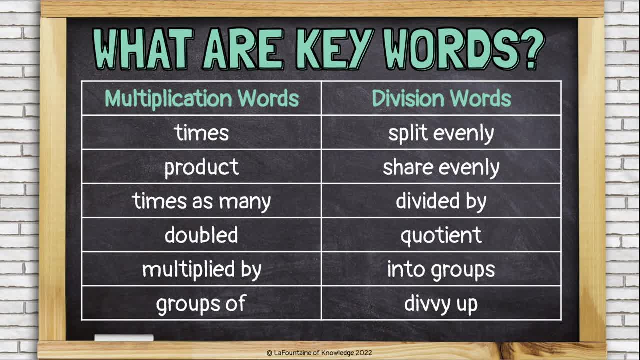 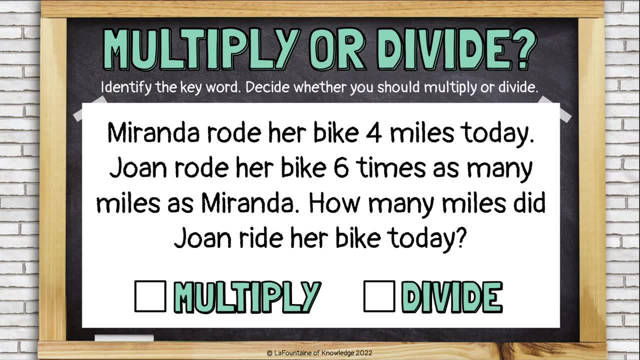 words might be split evenly, share evenly, divided by quotient into groups or divvy up. Let's see if we can find some keywords that help us decide how to solve a word problem. Keywords in this word problem: Miranda rode her bike four miles today. Joan rode her bike six. 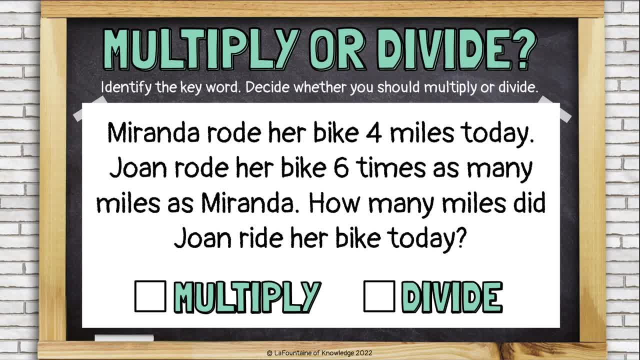 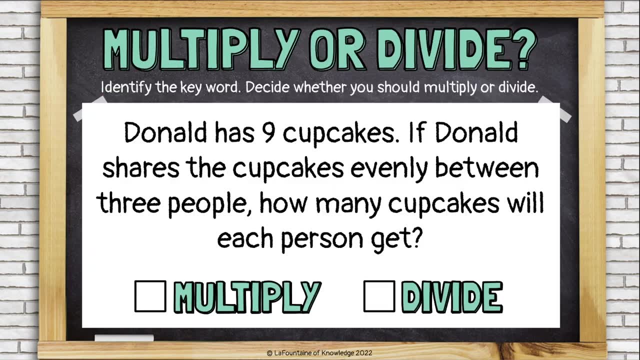 times as many miles as Miranda? How many miles did Joan ride her bike today? I see the keywords times as many. That to me means that I should multiply. Times as many usually means multiplication. Donald has nine cupcakes. If Donald shares a cupcake with his wife, he should multiply. 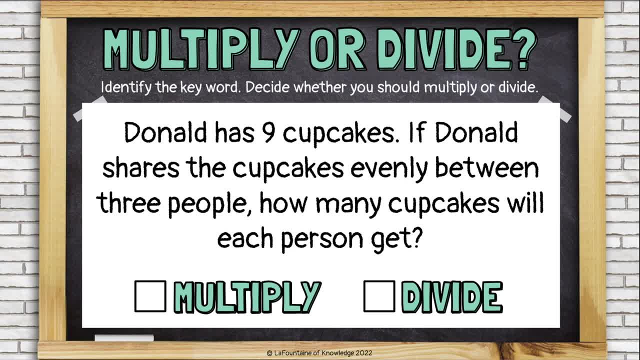 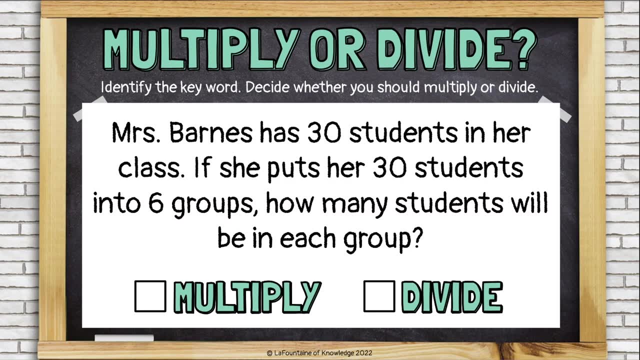 If he shares the cupcakes evenly between three people, how many cupcakes will each person get? Shares evenly: Those are division words. It means he's dividing up the cupcakes between those three people. Shares evenly usually means to divide. Mrs Barnes has 30 students in her class. If she 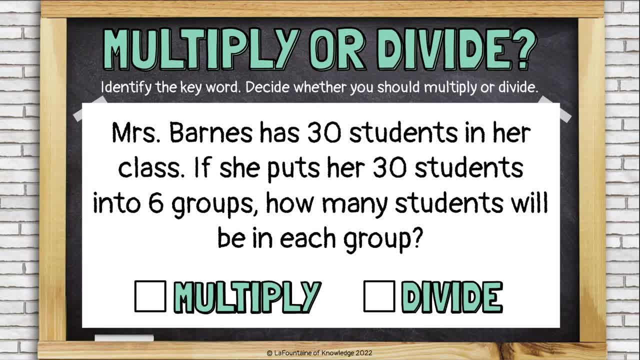 puts her 30 students into six groups, how many students will be in each group? Do you see any keywords here? Groups, That usually means to divide. But also, if we think about what Ms Barnes is doing, she's dividing up her 30 students into groups. Into groups usually means to divide. 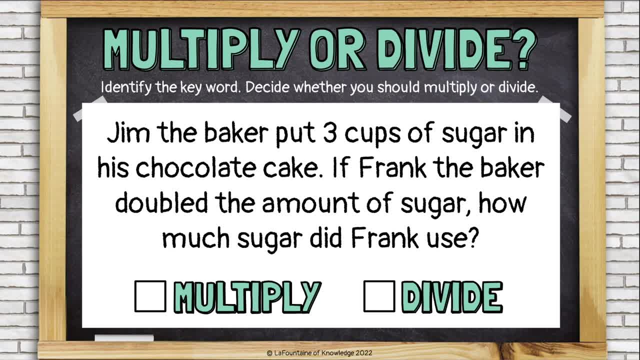 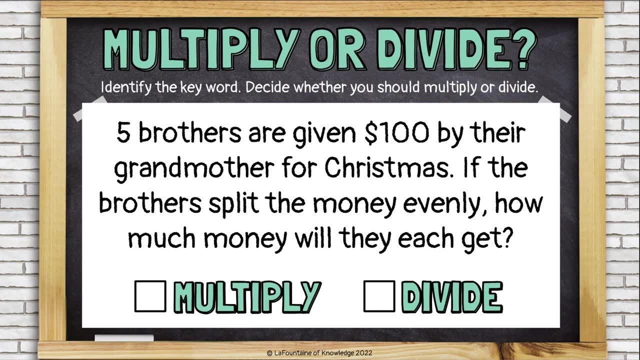 Jim the baker put three cups of sugar into his chocolate cake. If Frank the baker doubled the amount of sugar, how much sugar did Frank use? Hmm, Doubled. Doubled means times two. That's a multiplication word. Five brothers are given $100 by their grandmother for Christmas. If the brothers split the money, 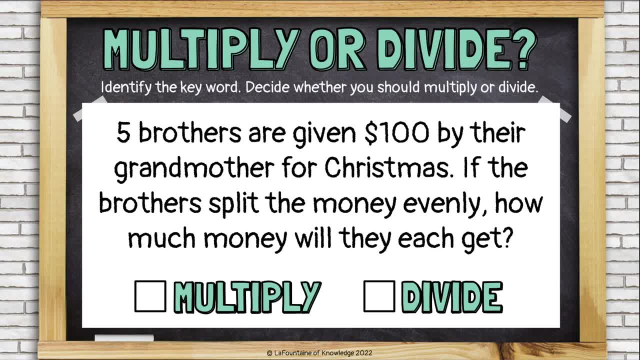 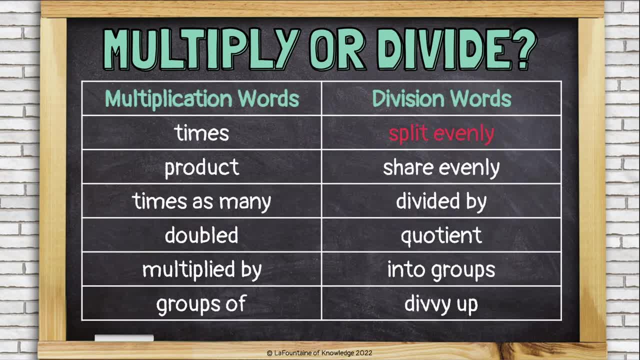 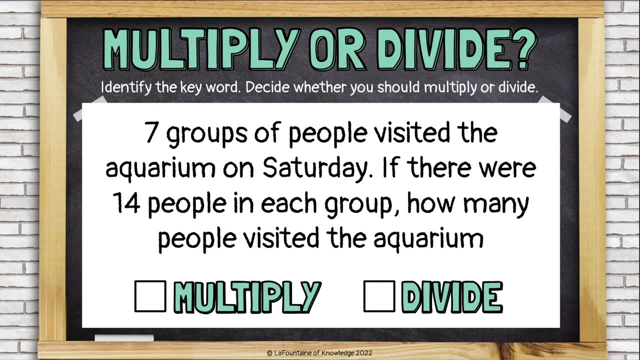 evenly. how much money will they each get? Here we have split evenly, which, just like share evenly usually means to divide. Seven groups of people visited the aquarium on Saturday. If there were 14 people in each group, how many people visited the aquarium? 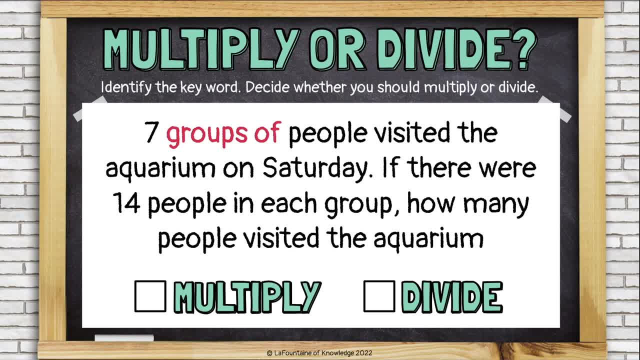 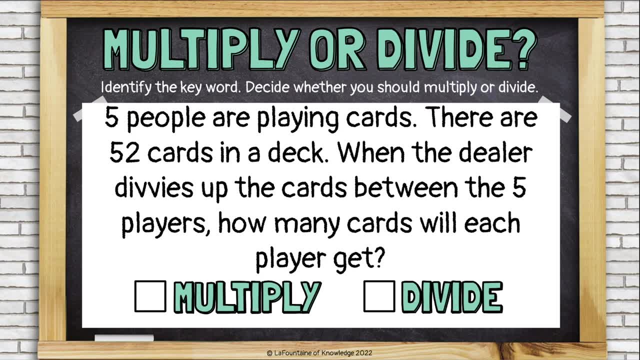 Each group Groups of, So we have seven people in each group. Those words suggest that we need to multiply. Five people are playing cards. There are 52 cards in a deck. When the dealer divvies up the cards between the five players, how many cards will each player get? Divvies up? You can.